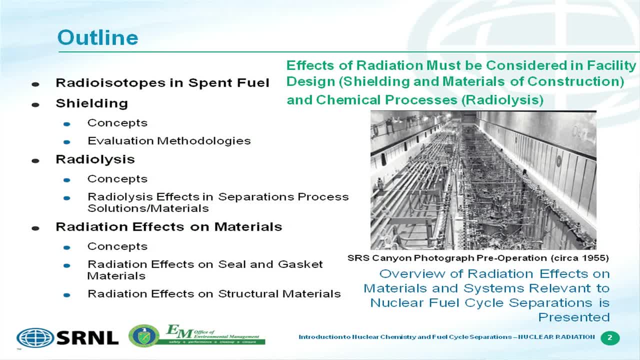 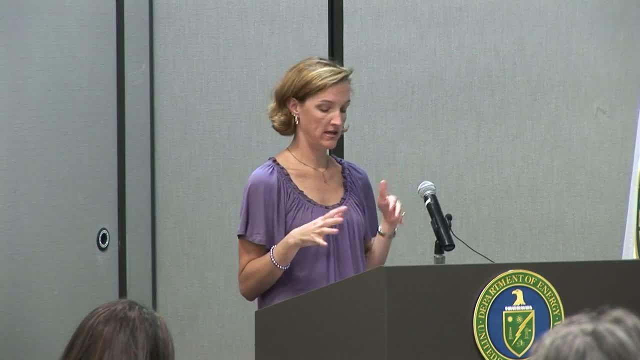 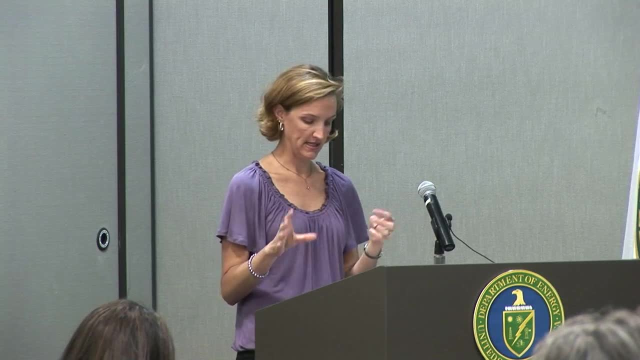 But I'm going to talk to you a little bit about the radioisotopes considered in spent fuel. You've heard about that for the past two days so we'll kind of quickly glance over it. Then I'm going to go in and talk to the three areas for consideration which are shielding for personnel, which is radiolysis and the effects that they have on the processing solutions and materials. 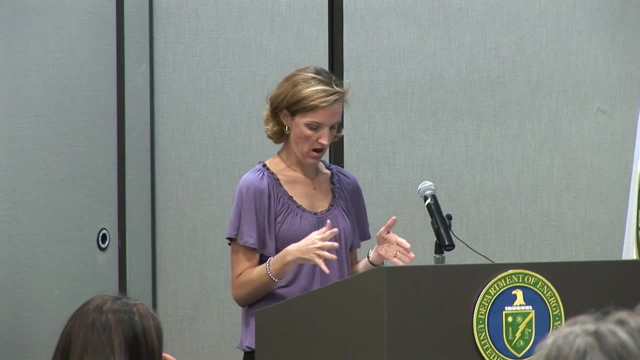 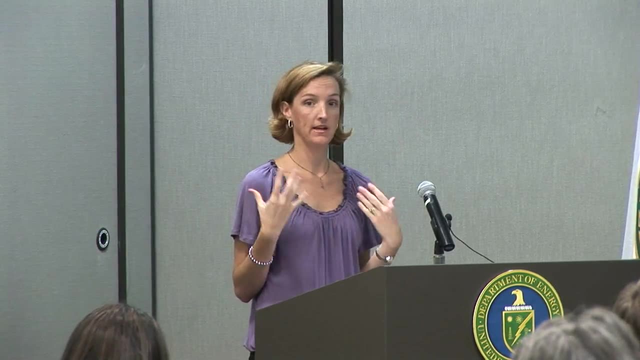 And then, finally, we'll talk a little bit about the radiation effects on the actual structural materials. As I said, this is a picture of our canyon. We have a lot of operating experience, with 60 years of experience of materials performance at the site. 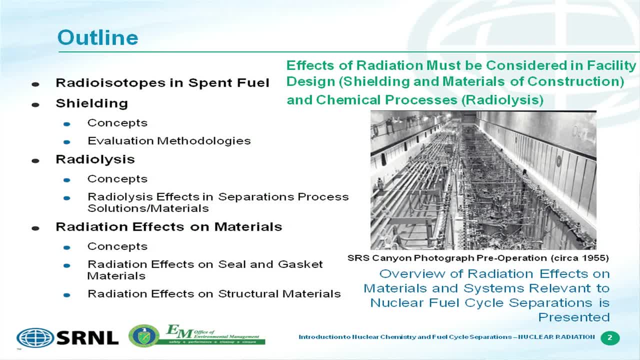 This is a picture of the canyon and you're looking at the north wall And from the right-hand side you get the cold chemicals coming in. They're brought in through the embedded piping on the right And then you see on the left-hand side – 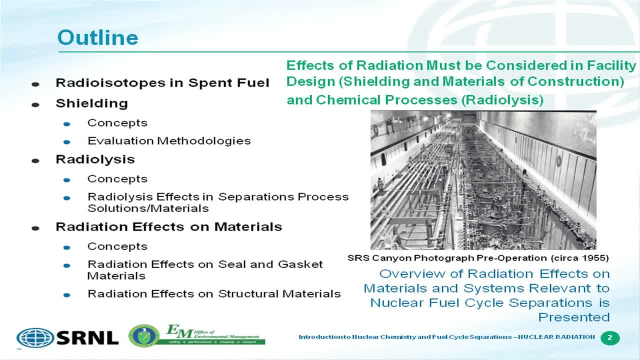 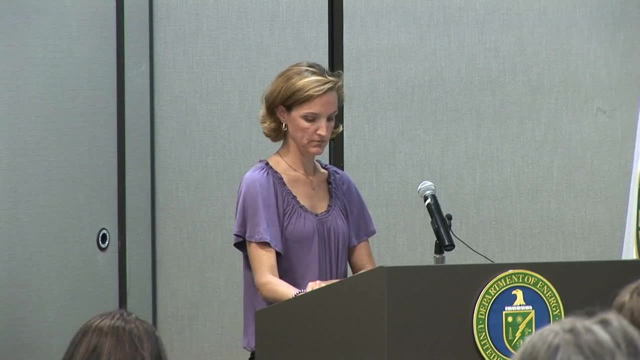 that's the hot wall for which the process liquids are transferred through embedded piping. You saw this picture – I think it was on Tuesday, I can't remember, But as you see, there's a lot of piping, and if all the cell covers were removed, you'd actually see the tanks of where all this process material is coming from. 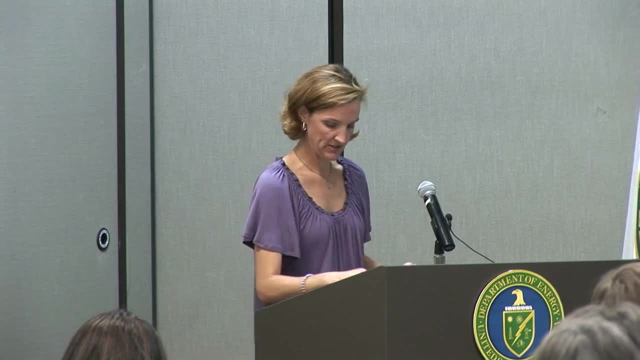 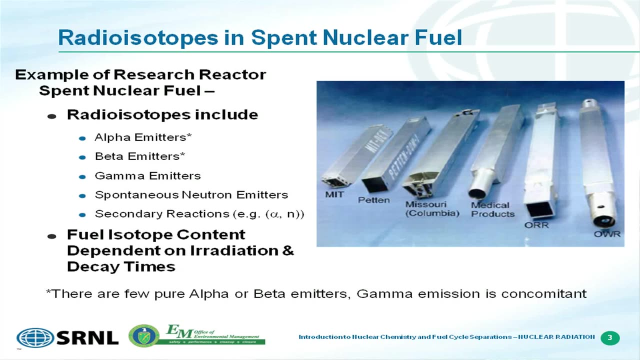 Okay to start off to discuss actually the source term of the radioisotopes in spent fuel. we're going to consider research reactor fuel and the isotopes following the operation of that fuel. So we're going to look at the source term of that and the discharge. 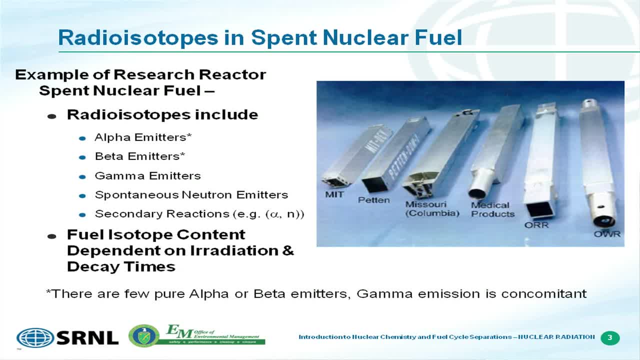 At the Savannah River site we have an inventory of over 11,000 materials, test reactor design and that is what that – oh, it's not up there, Sorry, I thought it was up there. And this is an assembly of a total of 15 to 19 fuel plates. They're each approximately 2 1⁄2 inches wide, by about 2 1⁄2 feet long, and they're about 50 mils thick. The cladding is also about 15 mils thick and the core is about 20 mils thick. 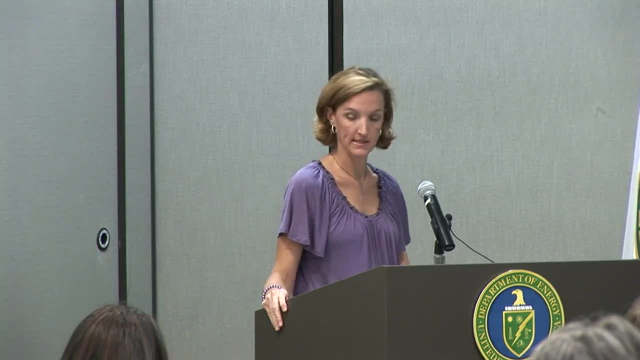 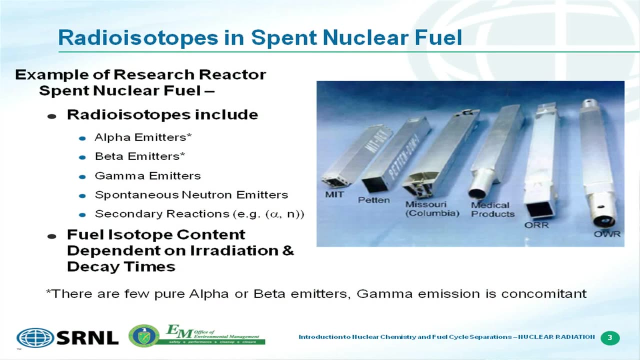 The cladding is nearly pure aluminum, It's an aluminum alloy and the fuel core is in a uranium aluminum alloy. As we know, what happens is the uranium fissions, leading to a suite of fission products, but we also get the absorption of neutrons, which is going to lead to a suite of actinides. 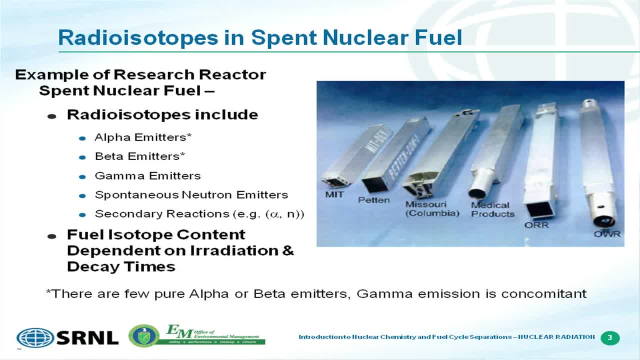 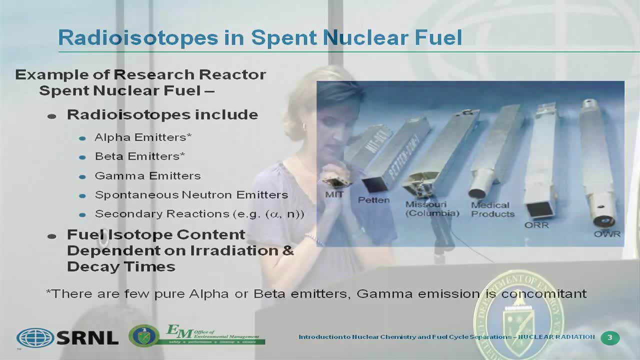 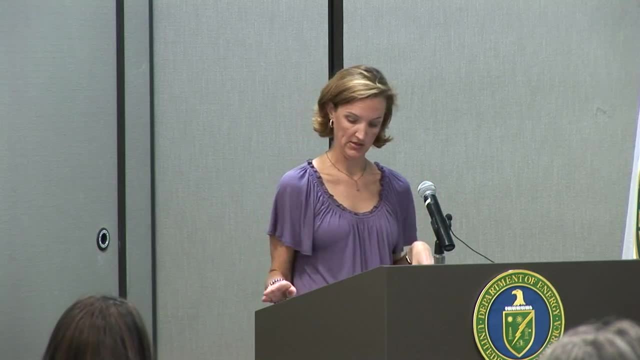 The radioisotopes produced. we can have alpha emitters, beta emitters, gamma emitters and we can also have spontaneous neutron emitters. Another source of neutrons is from secondary reactions, from the alpha neutron reactions considered like the amaryllium beryllium sources or the plutonium beryllium sources. 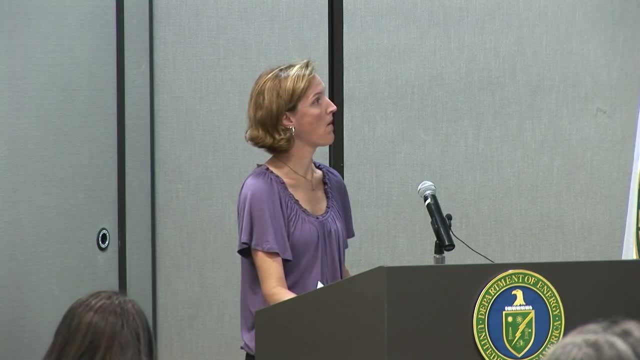 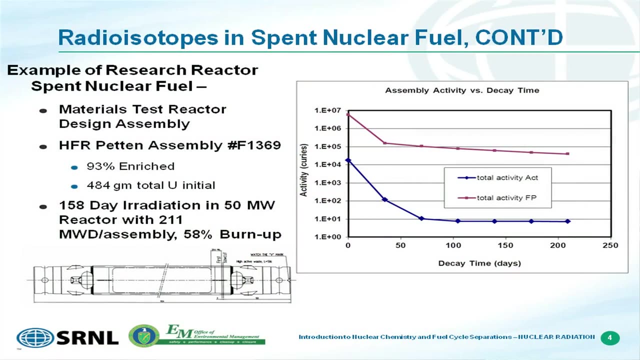 which are engineered as true neutron sources. Right now we can calculate the inventory of specific radioisotopes in the fuel, and this right here we're going to consider one of those MTR-designed fuel assemblies that was irradiated in the HFR Penton reactor, which is located near the Netherlands. 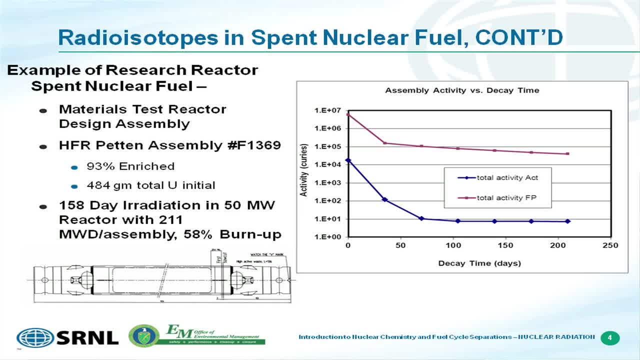 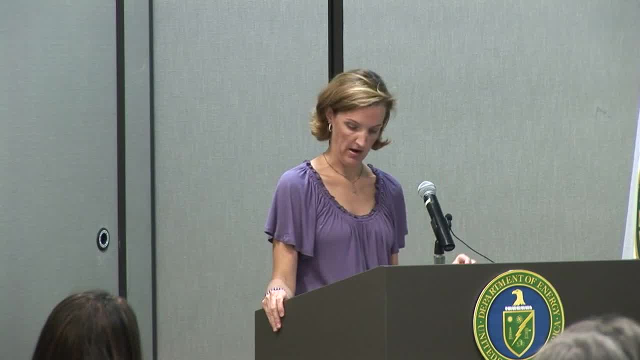 We can calculate this- the radioisotopes generated- either by building a model- We can do an assembly average model, a core average model or a 3D location-specific model. For the MTR case, we're going to consider assembly average model. 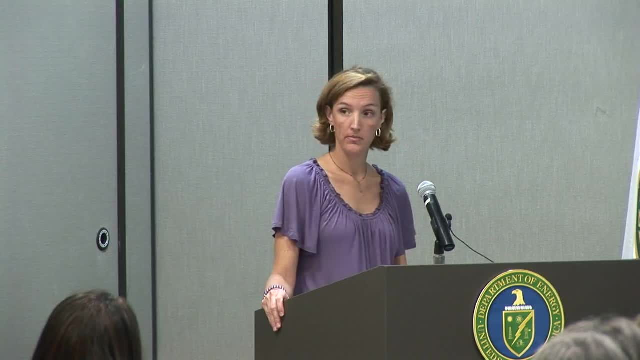 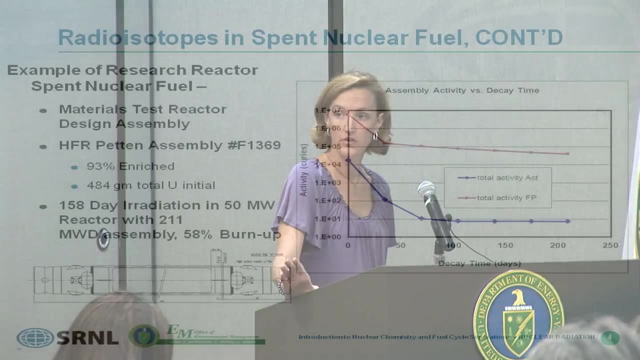 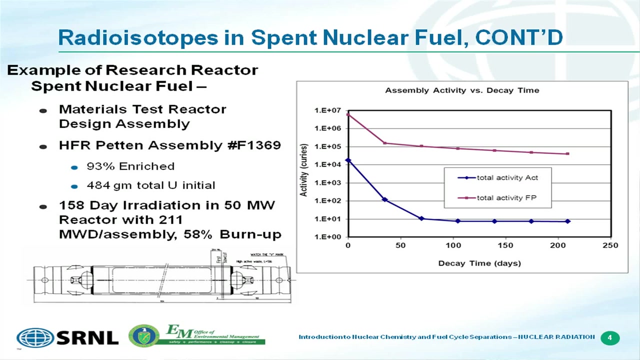 This fuel was irradiated at 211 megawatt days. That corresponded to about 58% burnup, which is that 58% of the uranium-235 species in the original assembly was irradiated. So that's the total amount of uranium that was fissioned. 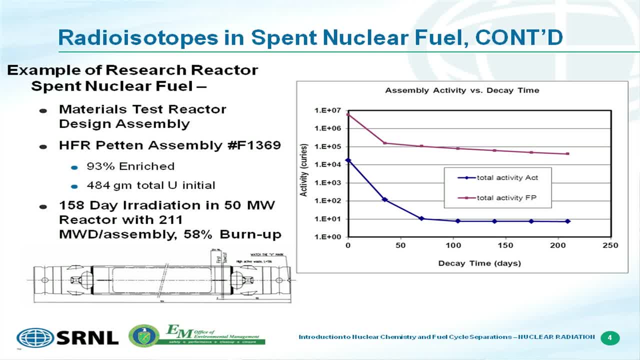 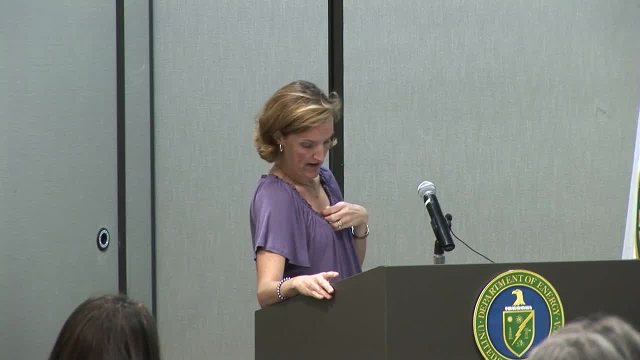 We can get an inventory of the fission products and the actinides that were created. As you see- the chart on the right-hand side- each group decays over time and we see well, not in this case, but after about a year of cool-down. 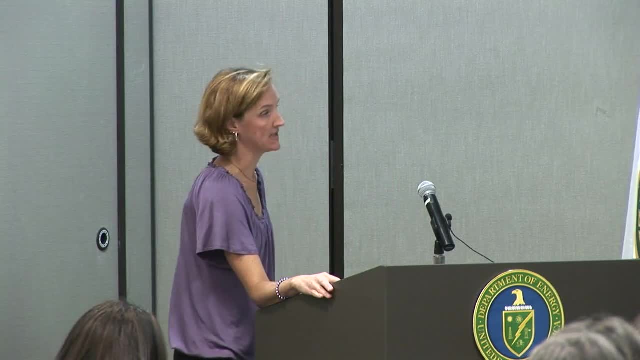 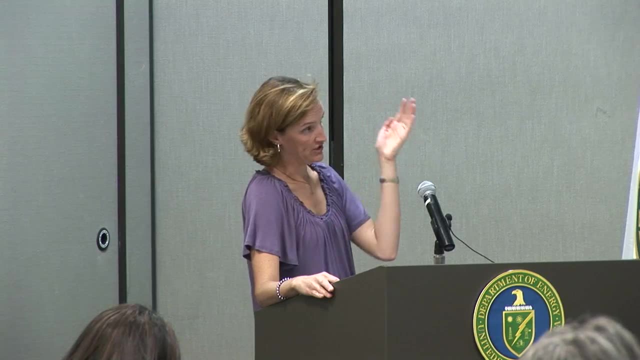 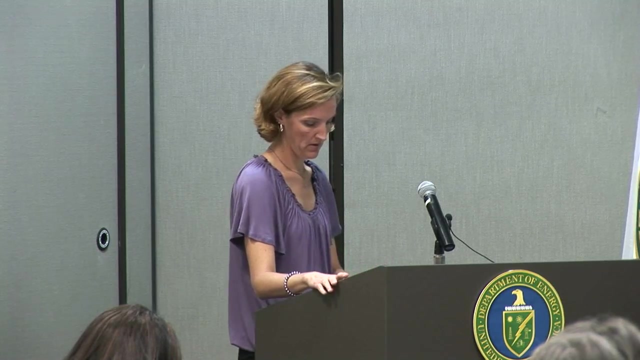 we're down approximately three orders of magnitude in the overall carrier activity content for the fuel that's dominated by the fission products. Also, as a side note, as the longer-lit- several hundred years cool-down, the actinides are the dominant species. 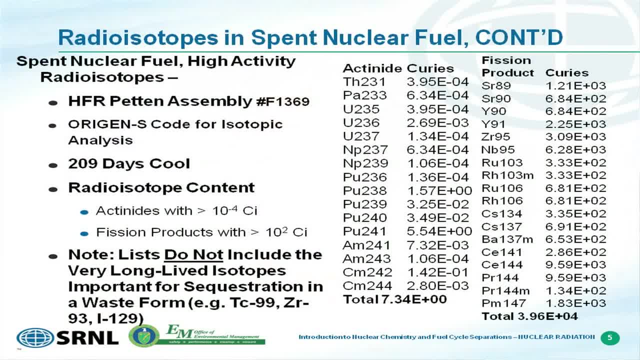 This slide shows the specific radioisotopes for the pentene assembly. This particular isotopic analysis was created using the ORIGIN-S code, which is a simulation tool that computed the actinide and the curie content. This was after 209 days of cool-down. 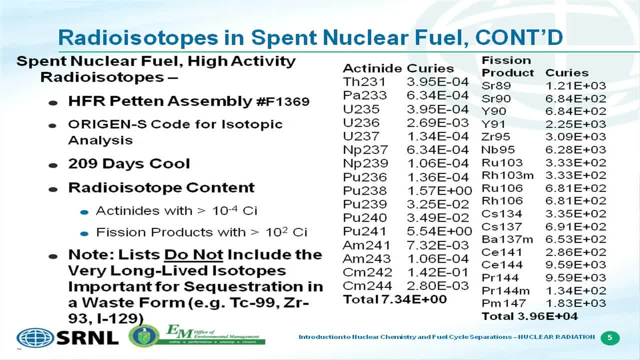 This was the last point on that previous slide- And for impact and shielding on the processing systems, you want to consider your highest activity. A listing could be developed for various isotopes that would remain for long-term storage or that would remain even for repository disposal. 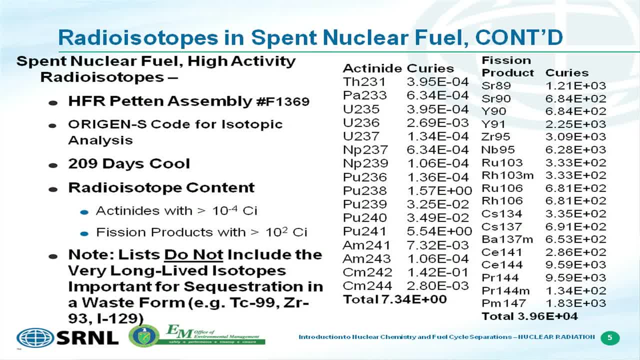 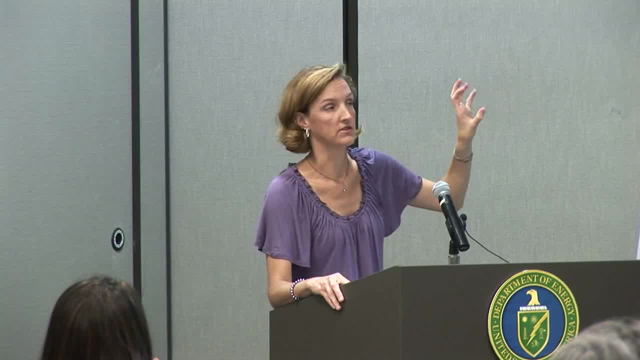 Right here, what we're seeing is the radioisotope content, the actinides only for greater than 10 to the minus 4 curie content and the fission for 10 to the minus 2 curie content, greater than 10 to the sorry 10 to the second curie content. 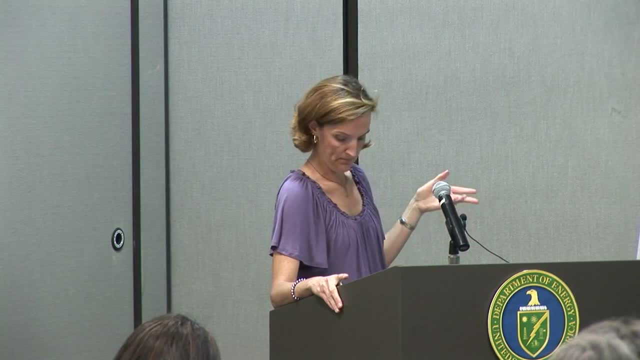 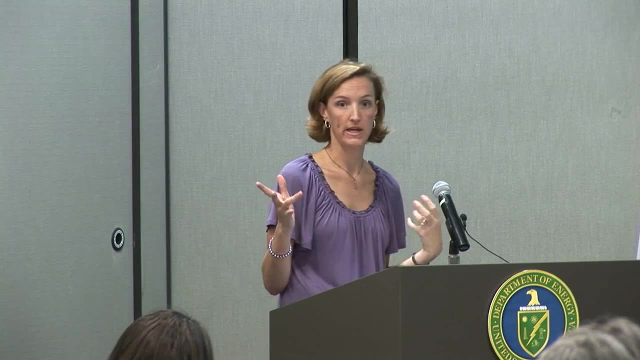 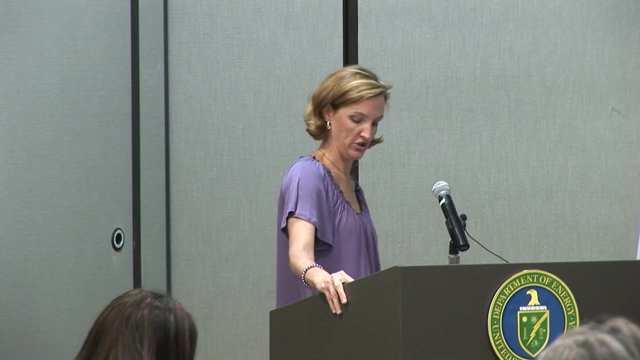 But there's others as well. We can also you know, as the listing activity is going to change with different time and with different isotopes. so we can design our, we can run our codes to find out the species that would remain for after separation processes. 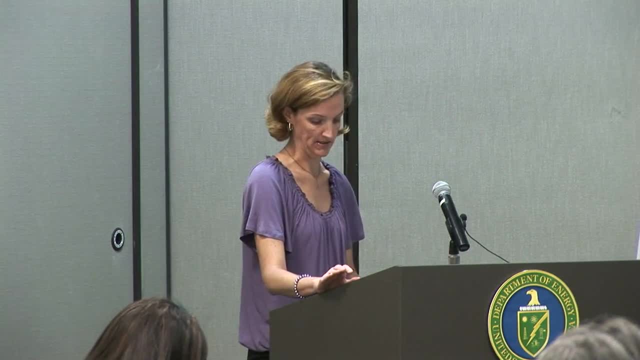 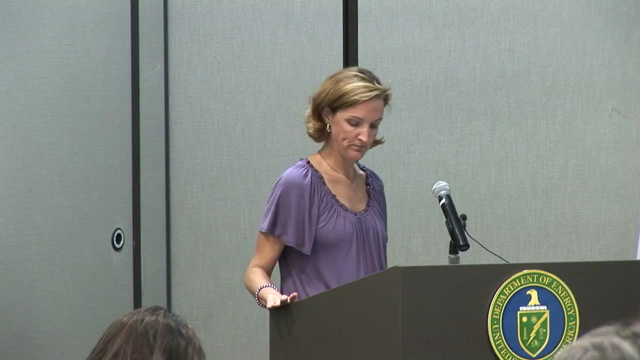 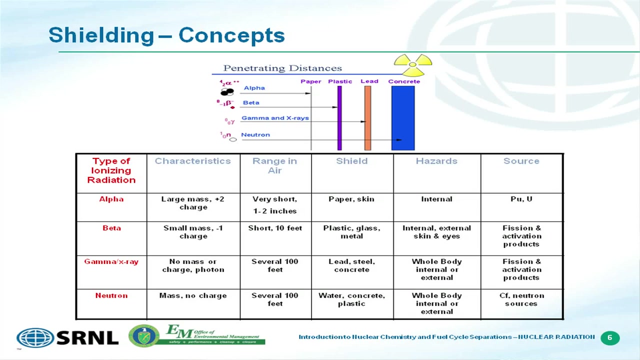 after dry storage processes or even repository disposal. Okay, now we're going to get into shielding. We all are, we all should, we should be able to design simple shielding systems based on our knowledge of alpha, beta, gamma and neutron radiation. 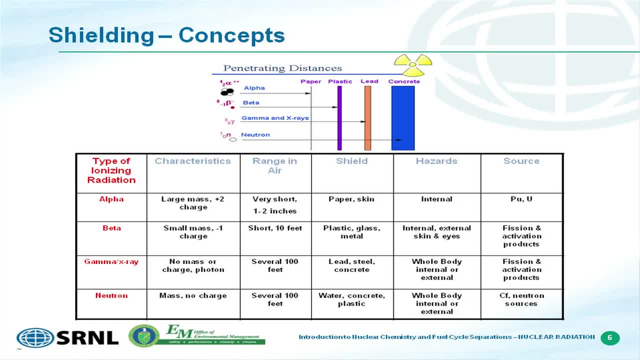 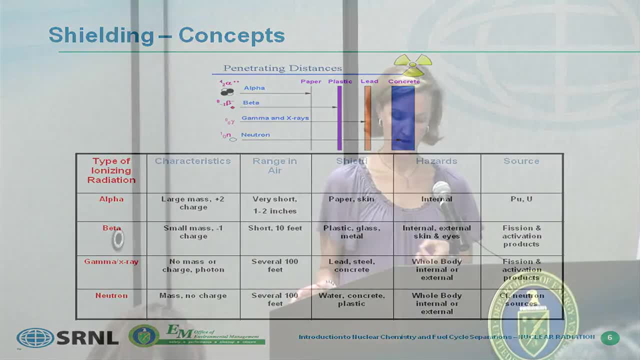 I'm not going to really go over this, just to but just to point out that gamma and neutron radiations we have to have other considerations in their shielding designs due to their long range in the air in an unshielded system. Whoops, sorry. 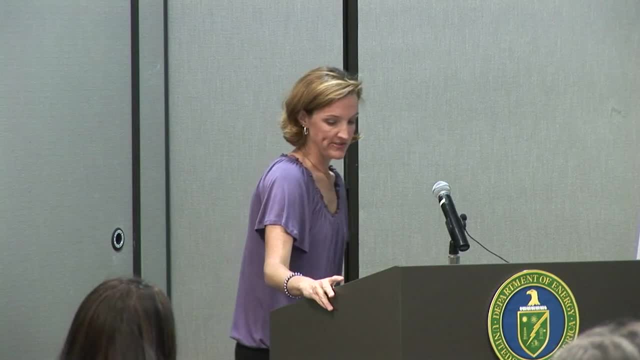 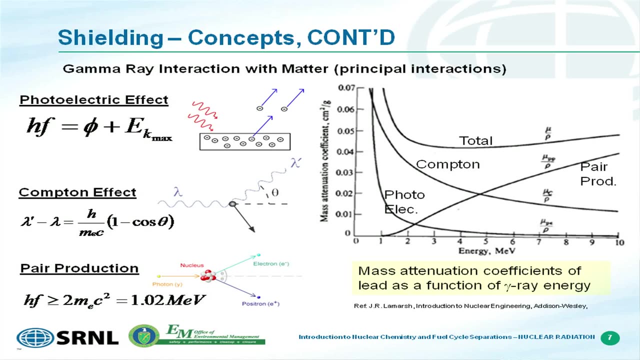 Trigger: happy, sorry. We're going to use gamma radiation to discuss the concepts of shielding. Gamma interacts with matter and it can be attenuated, so either it can be scattered or it can be absorbed in three principle modes. At low energies we have the photoelectric effect. 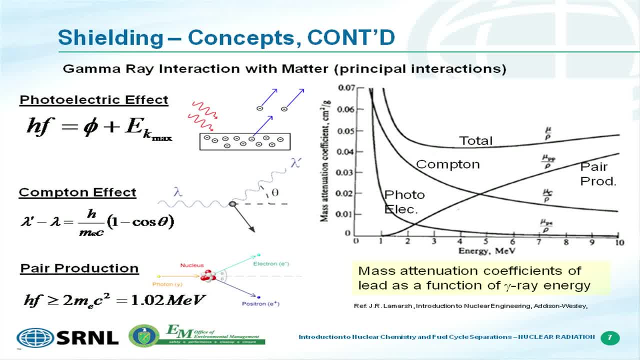 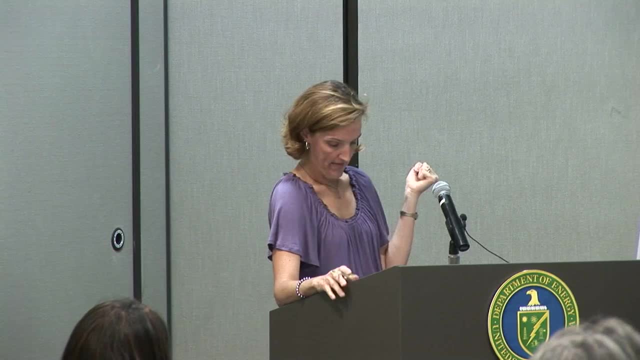 where a photon impacts and you get, or sorry, a photon imparts energy and the electron is shot out At immediate gamma energies. you get Compton scattering and that's going to produce a gamma at a lower energy in a Compton electron. 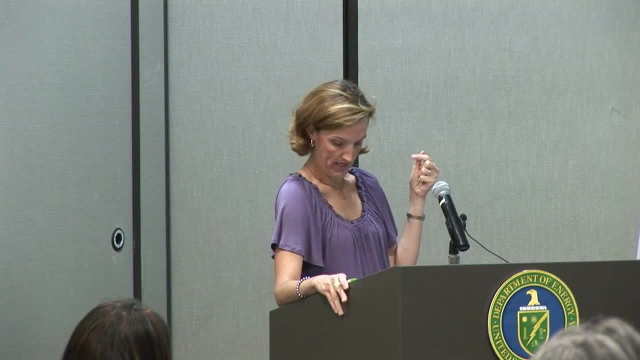 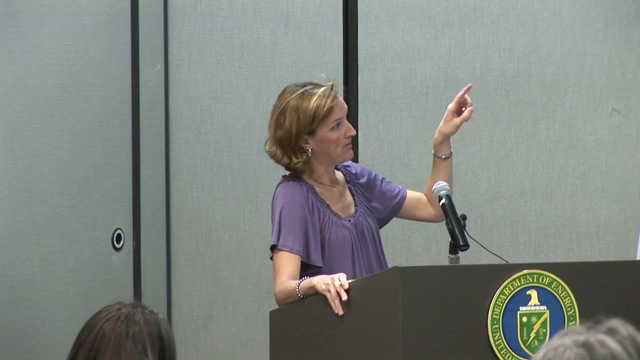 And then at higher thresholds, greater than one MeV, we can get this, the gamma pair production, which the gamma ray is annihilated, and then you get this electron positron creation. Now, immediately following that, the positron is annihilated. 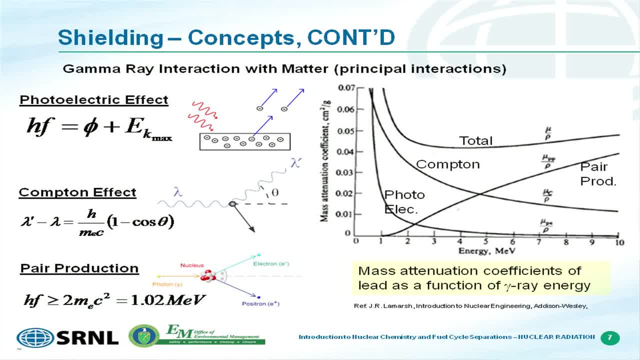 and it results in the formation of two gammas. This figure right here shows the attenuation coefficient for lead, which is normalized by its density For each of these interactions. the attenuation, which, if you remember, is the scattering absorption, shows as the incident gamma ray passes through the material. 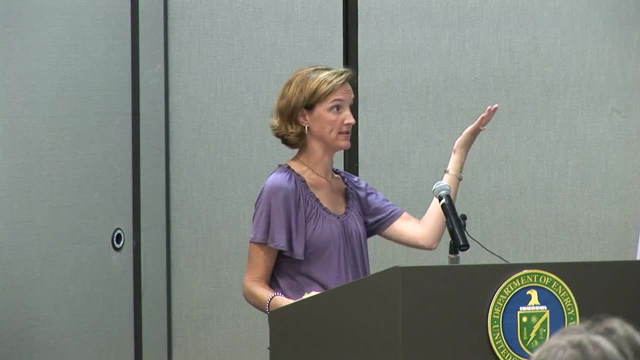 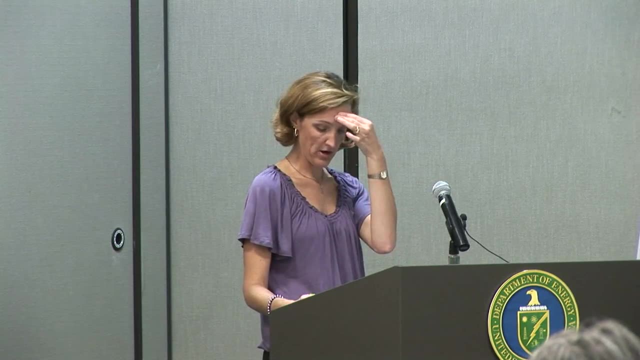 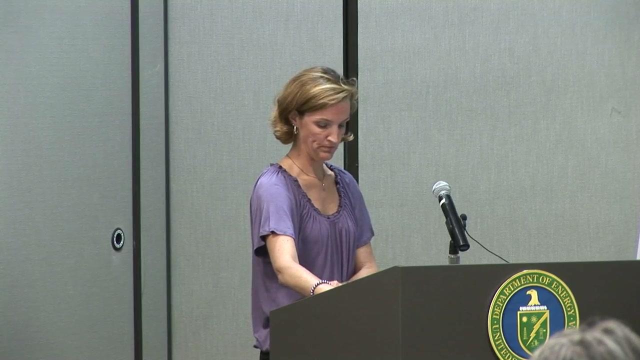 In this case the incident, gamma flux would be reduced by its attenuation coefficient. It's interesting to note that the energy deposited in a material primarily occurs via interactions to produce electrons which slow down in the actual absorber material. Okay, now to talk about shielding again. 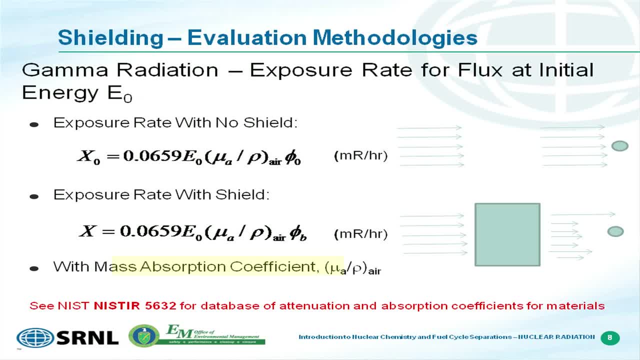 with exposure rate for flux out of an initial energy. This is when we have an emergent gamma. flux is absorbed in a mass of air. So let's say this point over on the right-hand side Now, in the case of no shielding or no attenuation, 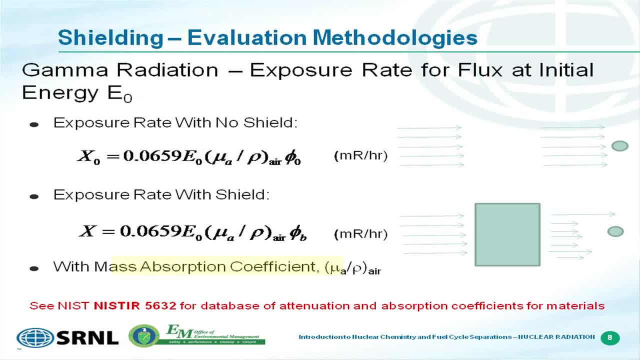 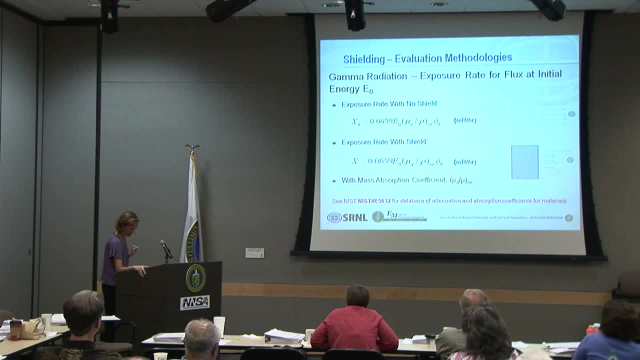 of the flux of gammas. the exposure rate is going to be correlatable to the flux of gammas. The flux of gamma is going to be correlated to the flux of gamma, So the incident energy as well as the mass absorption coefficient for air. 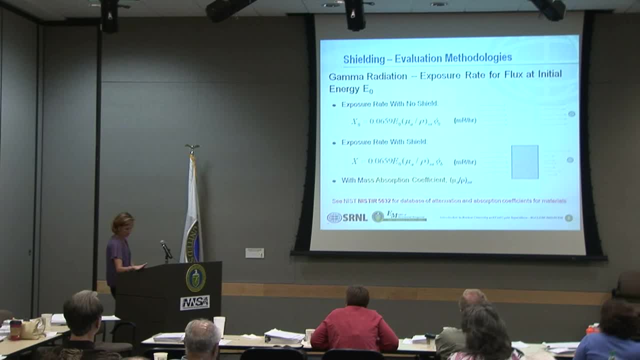 Now, with a shield, you get this buildup flux results and you have the construction of a buildup flux and we have that. That buildup flux is made to enable simple engineering calcs for the exposure rate in our volume of air after the gamma has been altered in its spectrum. 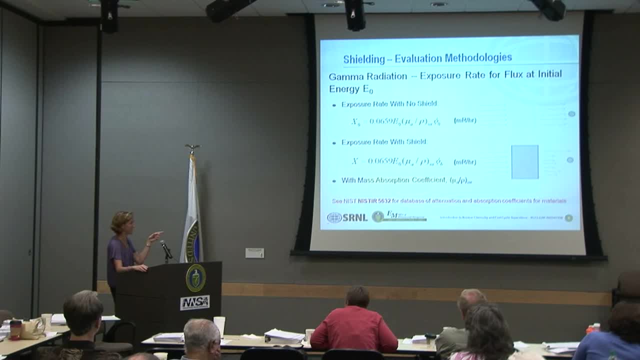 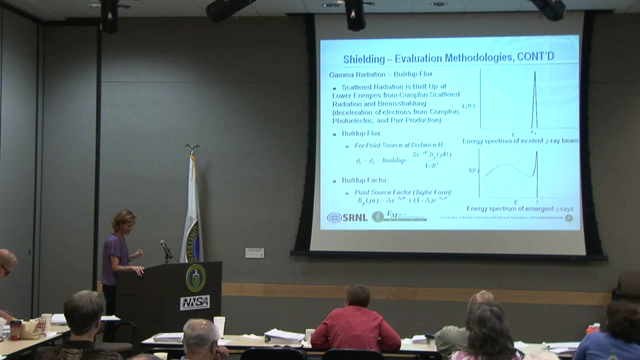 by passing through that shield. This does provide a database of various attenuation and absorption coefficients for a wide range of high to low to high Z materials compounds. Now, with this buildup flux, this the. I've got to watch what I say. 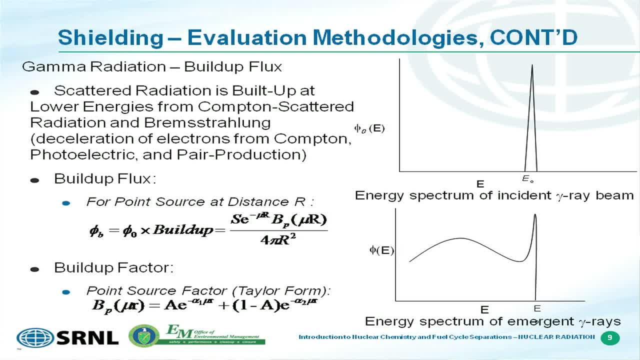 The figures on the right show the concept of the alteration of that initial gamma energy spectrum after it passes through the shield material. That top shows the incident energy. The bottom one shows that although the incident energy peak has been reduced, we have this buildup of flux right here. 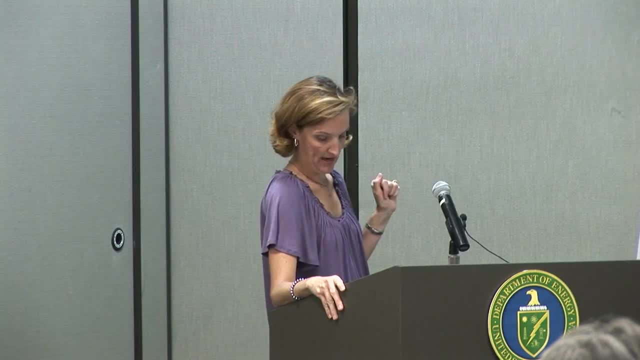 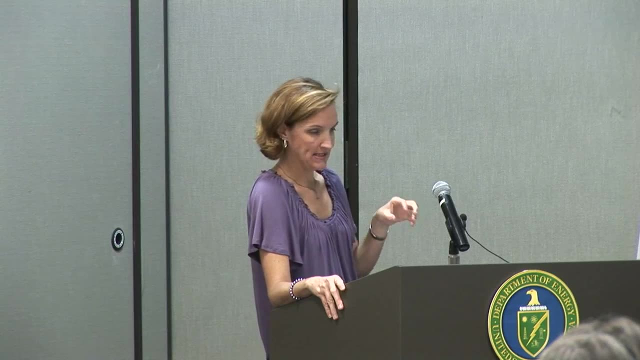 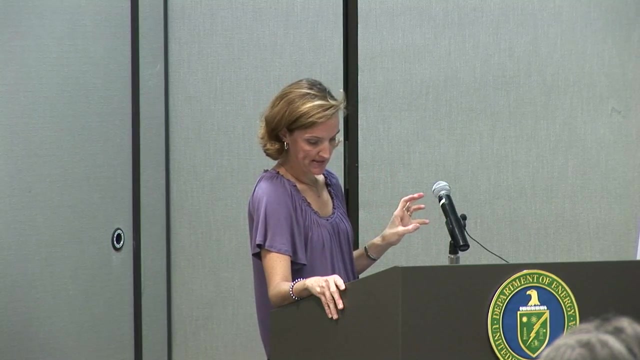 and that's a lower energy gamma that's built up. Now. the buildup factor that we have to take into consideration correlates the attenuated flux to the integrated flux, including the flux at the lower energies. You can look up these in tables and text. 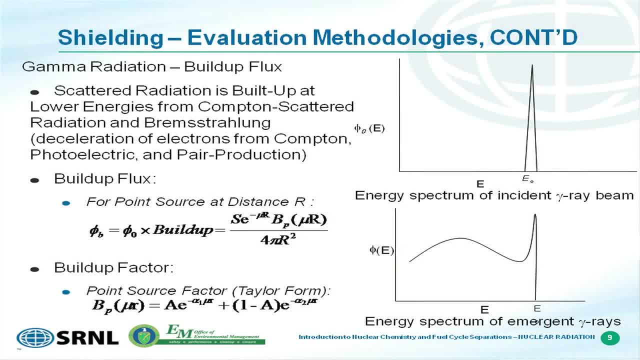 and use it in the following, in all these formulas, to calculate what that buildup flux is. Now, if we, It'd be very easy to compute a flux if every time the photon interacted with matter, it just disappeared. but it doesn't do that. 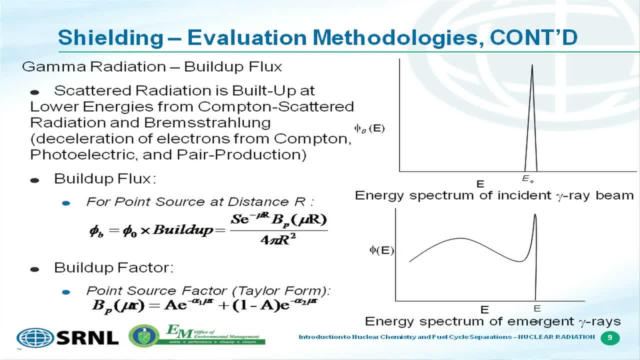 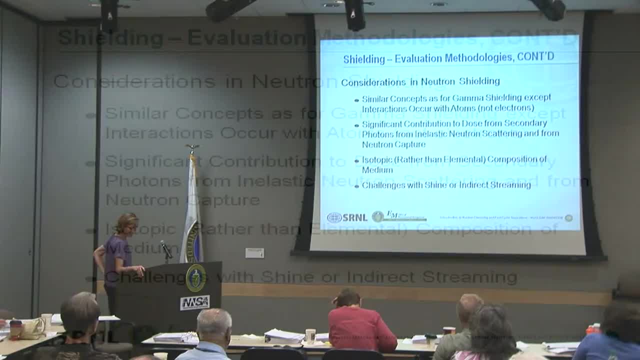 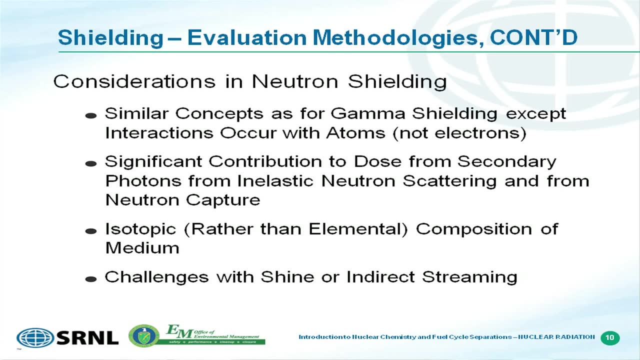 so we have to take these flux, these gammas, into consideration. Now, neutron shielding is a little bit different. It's similar, except that the primary interactions of the neutrons are with the atoms of the shield material. The complexities arise due to the creation of a gamma flux. 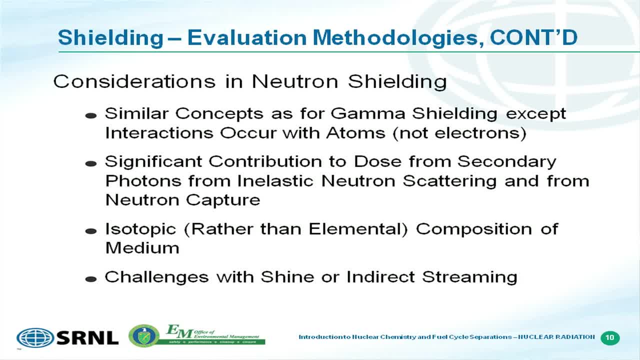 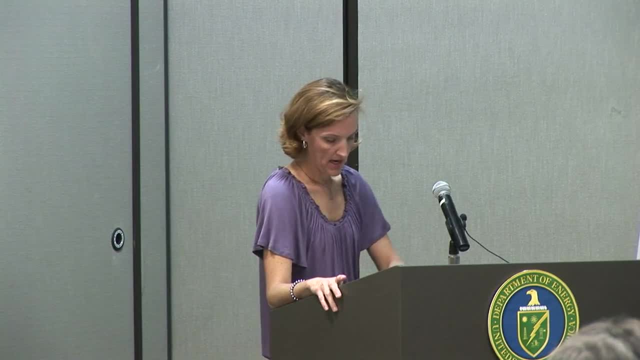 from the scattering reactions with the nuclei, as well as from neutron capture reactions, and another thing that you need to consider is the isotope of the shield for neutron capture reactions. Now we can use those formulas on the prior page to calculate what our buildup flux is. 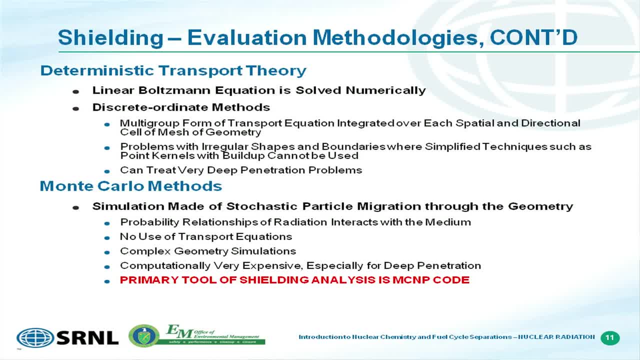 but for higher accuracy. we want to move on to transport theory or Monte Carlo methods. These are typically for the tabulation of factors for particle energy and shield geometries for flux buildup. Because they're limited in that previous formula, we have to go to these. 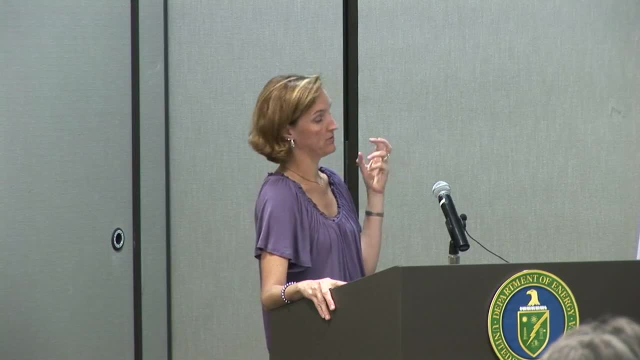 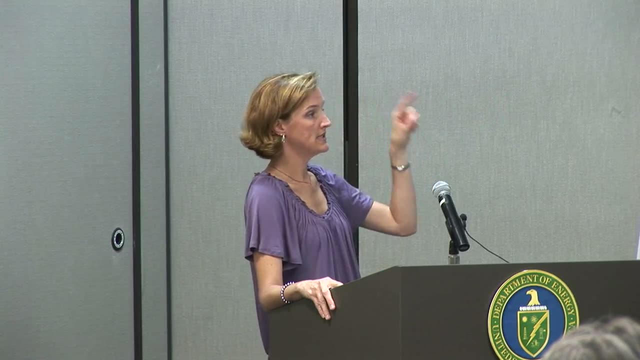 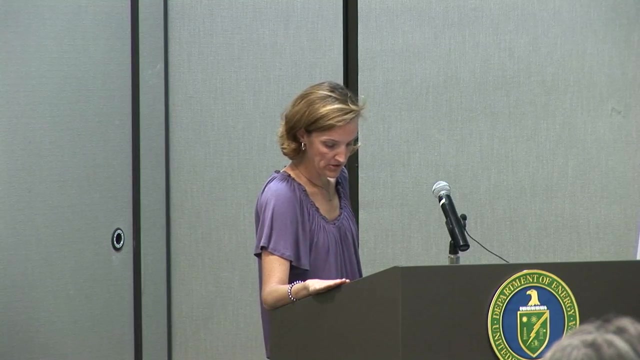 The primary tool of analysis when we want to sharpen our pencils to the greatest extent is the Monte Carlo method, and the Monte Carlo n-particle code is the tool of choice for these applications. but just a reminder that all of the canyon facilities were not built on the Monte Carlo methods. 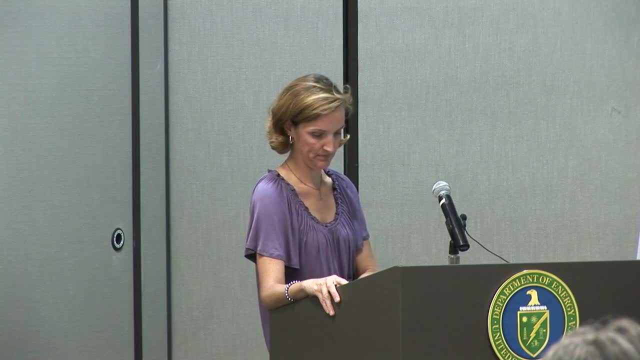 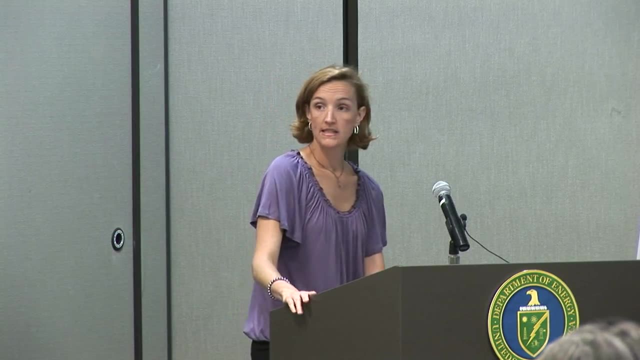 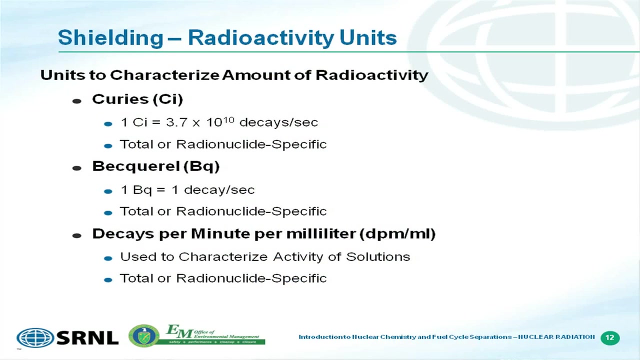 They were built on those simple calculations that we saw up front. Some units to characterize the amount of radioactivity- You've all seen these before, but what you'll see is the curies- and that represents the total or its radionuclide specific. 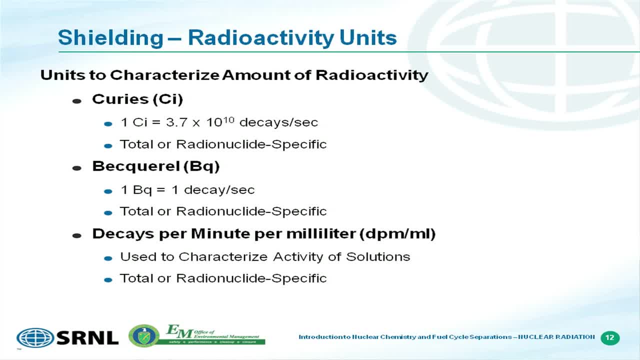 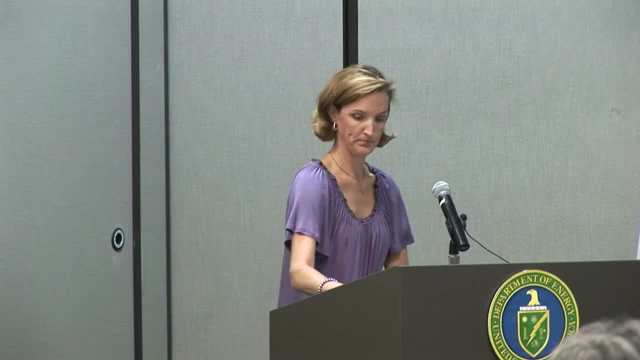 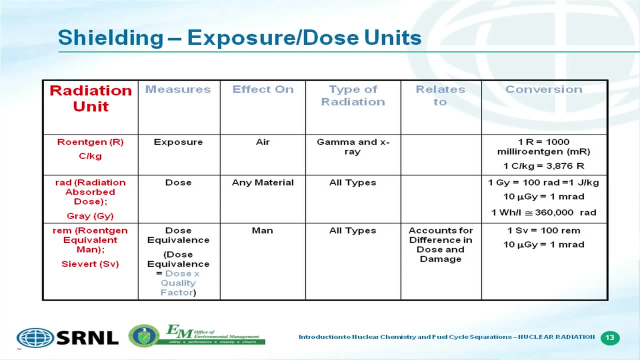 as well as the Becquerel. The decays per minute, per milliliter are used to characterize solutions and you can also find that in Becquerel per mils For exposure dose and dose equivalent units. they're defined in this table. 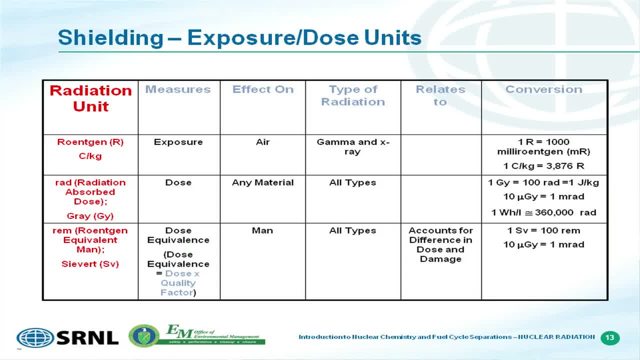 The Rankine is the unit of exposure that relates to charge production in air. It's rarely used as a practical parameter. Dose is the energy absorbed in a unit mass. In DOE we use the rad. that's equivalent to one joule per kilogram. 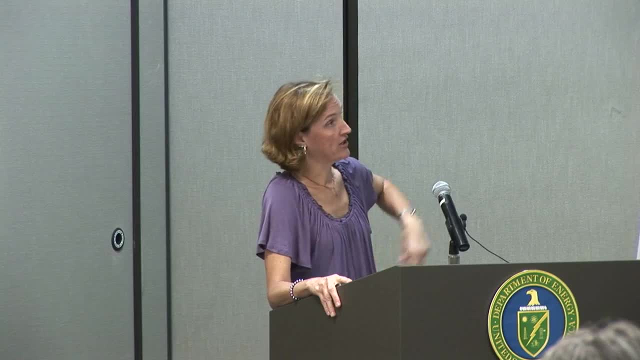 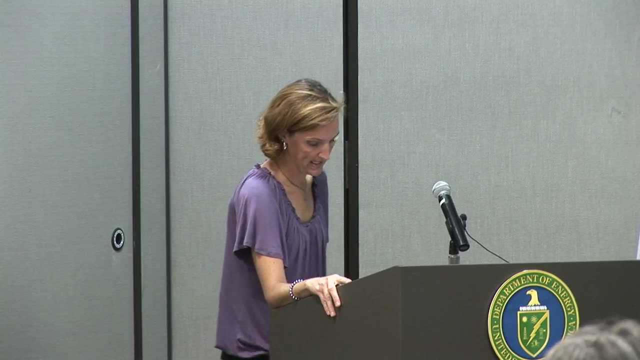 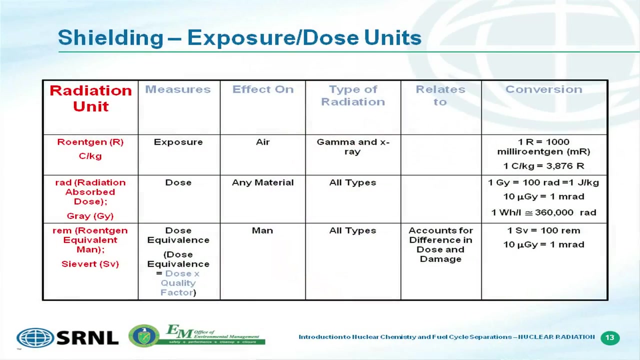 to express a radiation dose. The standard international unit is the gray and that is equivalent to 100 rads. When we want to take the dose equivalent, the last one here is a unit that includes a factor to weight the energy disposition concentration effects. 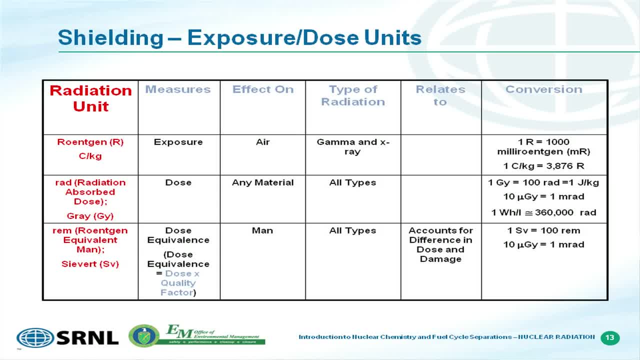 and that is the rem. Basically, when you have different radiations and different types of energies, that's when you use this and this. The SI unit for that is a sievert, and one sievert is equal to 100 rem And I believe that bottom equation. 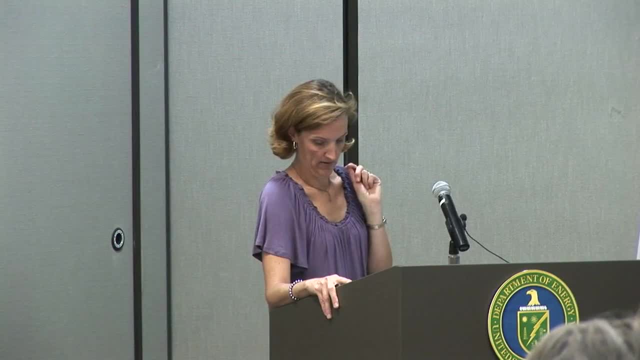 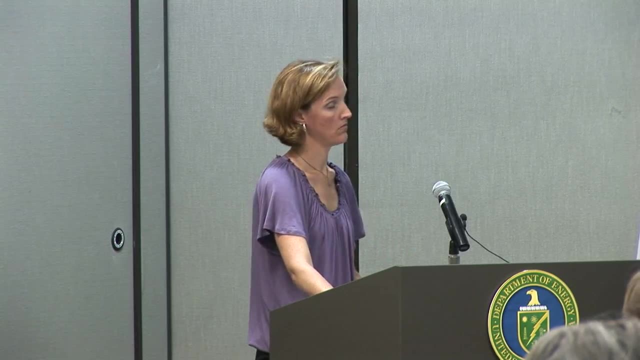 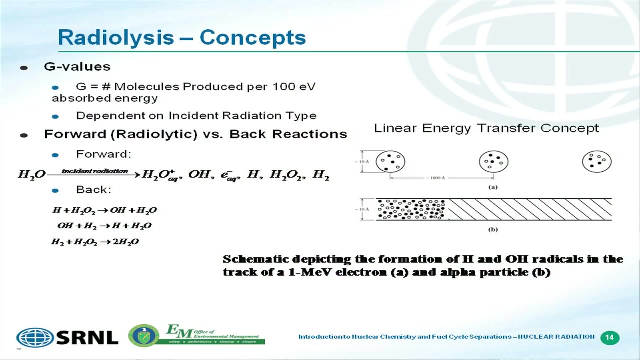 should be: one micro sievert equals one millirem, not gray and millirem, so sorry about that. Next we're going to move on to radialisis. Radialisis of the material is characterized as the production of compounds into its incident radiation. 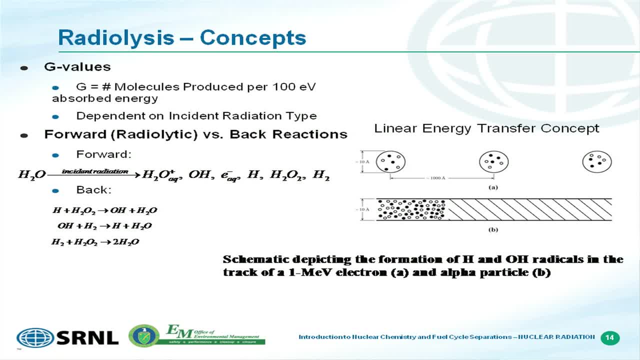 The conventional parameter used is the G value, which is the number of molecules produced or destroyed per 100 eV of absorbed energy, And the products that are created are very, very dependent upon the incident radiation. We're going to look qualitatively. 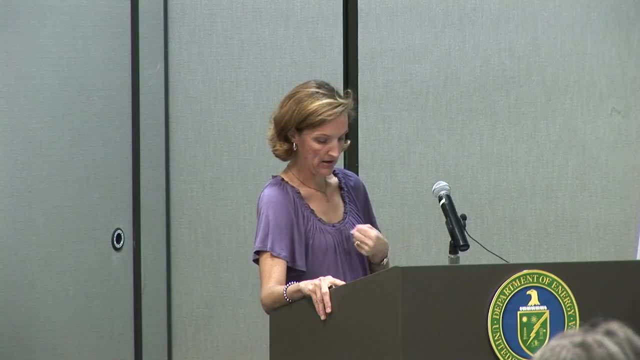 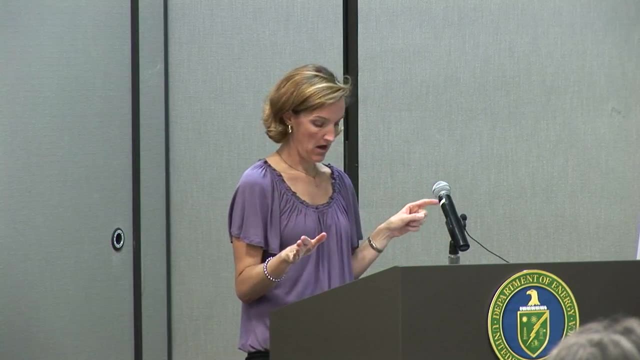 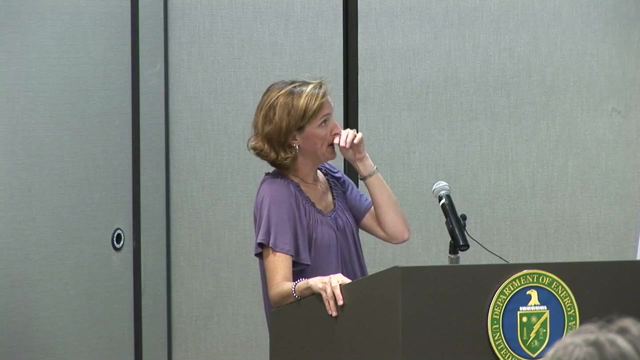 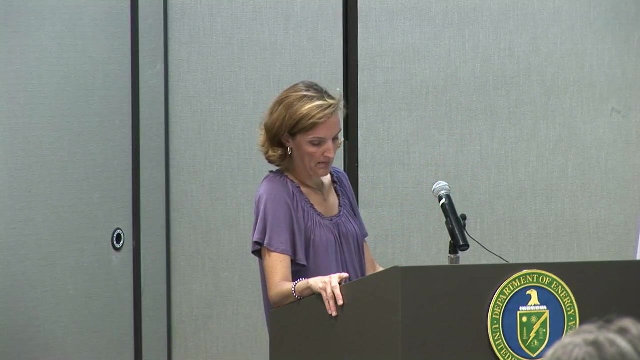 at the production of free radicals and stable compounds from the radiation interaction as energy is transferred to the system. A typical example here is water, And we see water when incident radiation hits it. it breaks the part into a bunch of different components. These are the overall chemical action. 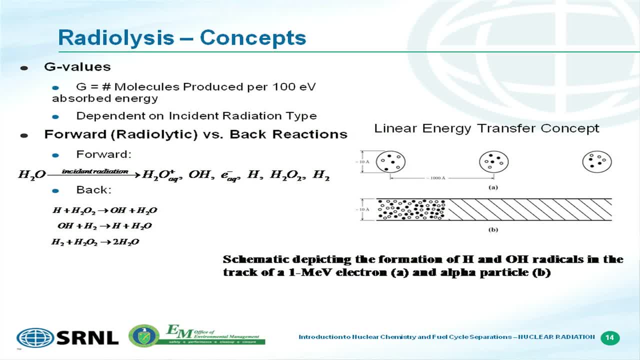 of radiation in water that you can find. You also can get back reactions when you have the hydroxide, or reverse reactions when you have free hydroxide and hydrogen radicals and they're interacting with other species and they create water again. A strong forward reaction to produce new compounds occurs when the molecular yield is greater than the radical yield, and the observed G value for a system is a net result of all of these reactions. For water, the G value is actually 4.5.. 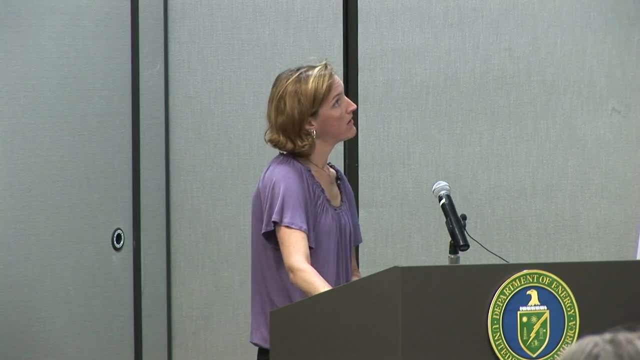 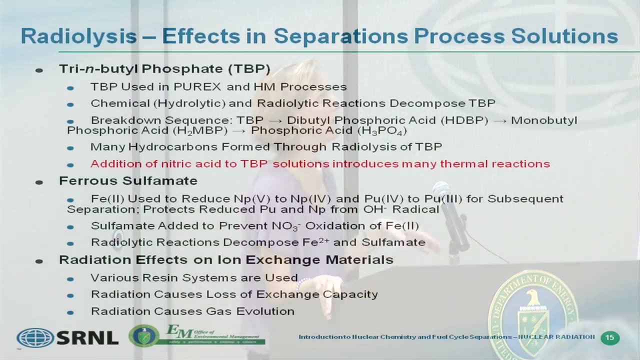 By gamma rays. that is Next. we're going to talk a little bit about the effects of radiolysis in separation chemistry systems. The first two we're going to deal with aqueous process solutions, and then the third is going to talk about 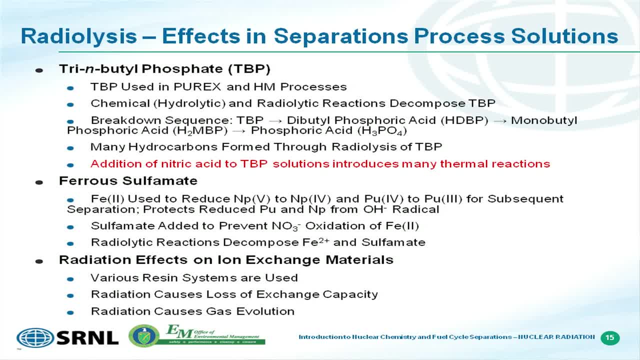 the exchange materials for these systems. As we heard Tuesday and Wednesday a lot about TBB and its use in the PUREX and the HM processes. Chemical and radiological reactions do radiolytic- Sorry- reactions do decompose the TBB. 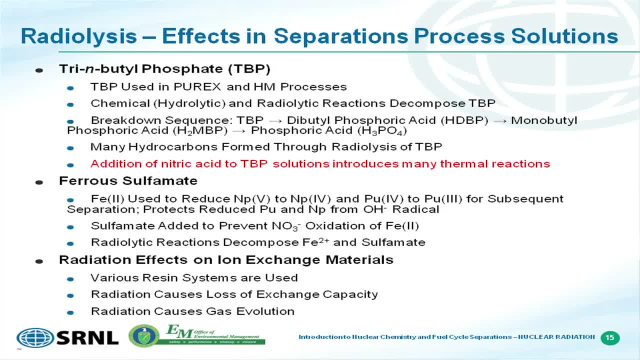 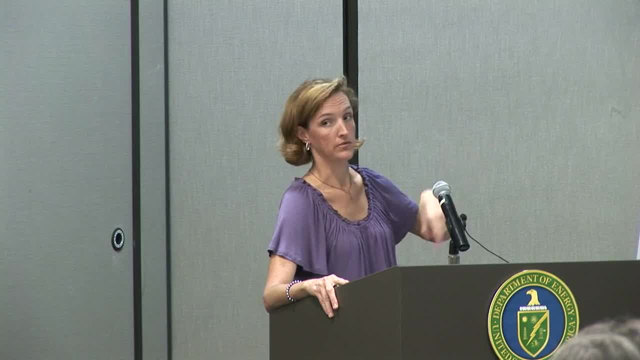 and the breakdown sequence for TBB, as we heard, also goes from the tributyl triambutyl to the dibutyl phosphoric acid, to the monobutyl phosphoric acid and then to phosphoric acid- Some of the various degradation products. 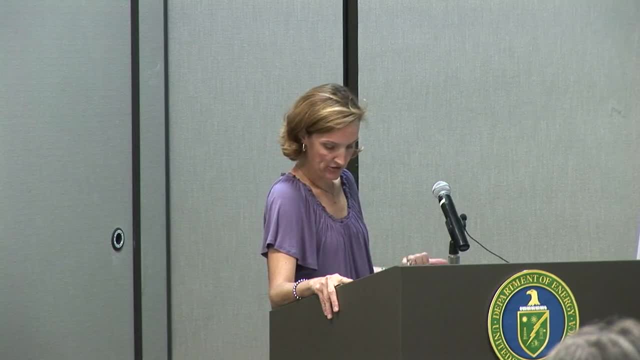 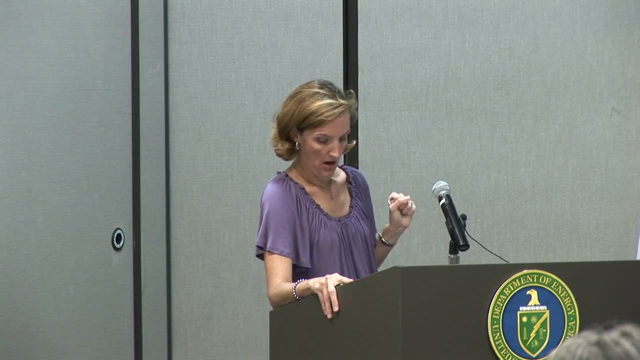 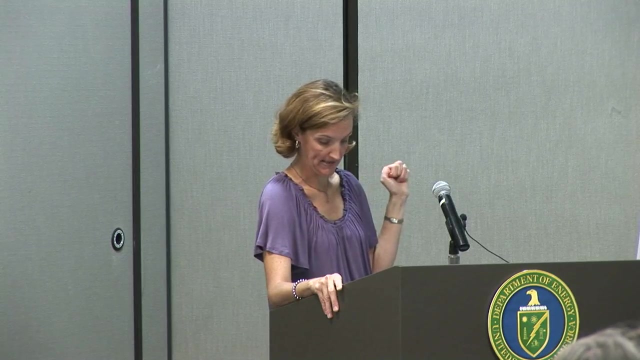 that are produced are those, as well as hydrogen, methane, ethane, various hydrocarbons and even polymers are created from this degradation. Also, addition of nitric acid to the TBP solution does introduce many thermal reactions as well. You heard, first, sulfamimate is used. 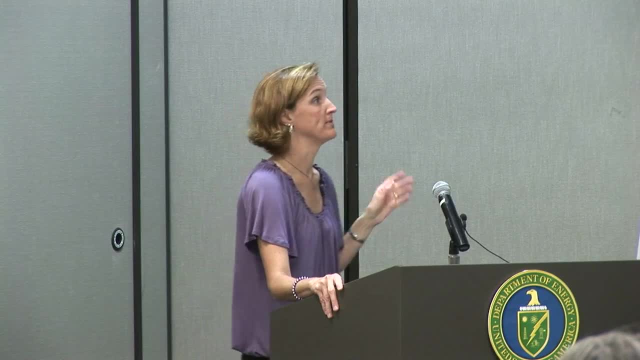 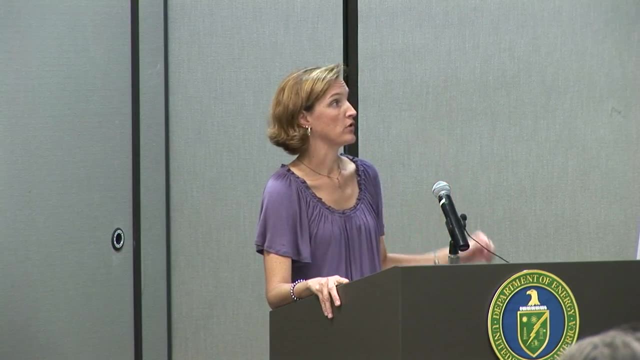 to reduce the neptunium-5 to neptunium-4 and the plutonium-4 to 3 for separation, and what the iron is used for. to protect those forms from the OH, radical Sulfamimate is added to prevent. 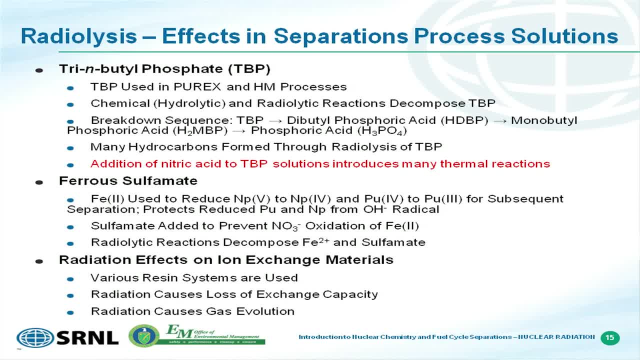 the nitrate oxidation of the iron-2, and when you get interaction with radiation they decompose both that iron and the sulfamate. Radiation effects on ion exchange materials. Various resins are used in systems, as we heard, You can, when radiation the effects of this. 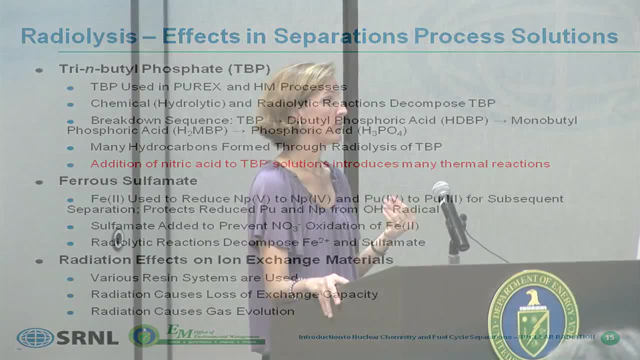 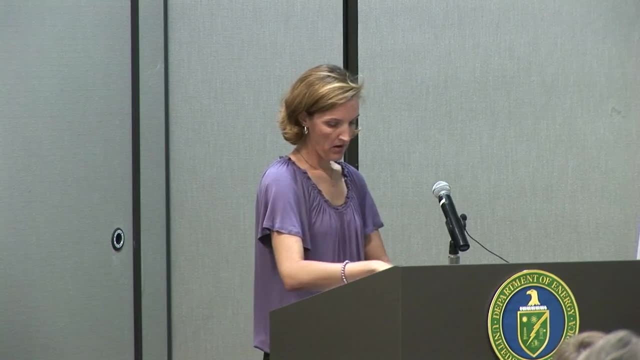 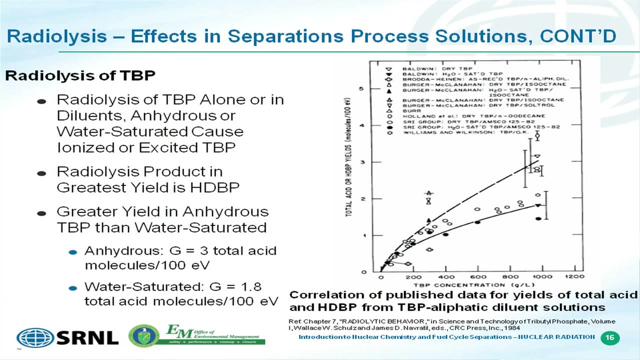 are loss of exchange capacity with those resins, as well as possible gas evolution. The radiolysis of radioactivity of TBP is very dependent on the solution that it's in, However, in all systems the dibutyl phosphoric acid. 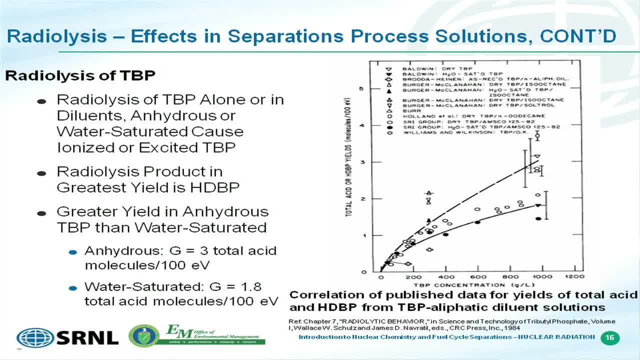 is the primary radiolytic compound. This chapter on radiolytic behavior. it provides a very, very good analysis of all of this radiolysis effects observed on TBP in various forms. This particular graph was taken out of that and it shows that we see greater yield. 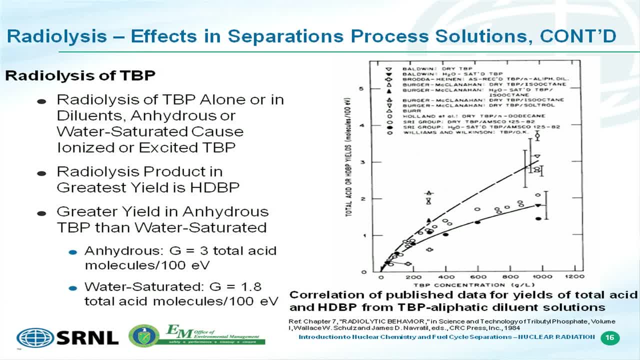 of total acid, or HDP, in anhydrous TBP than we do in a water-saturated TBP. What this is is TBP in various aliphatic solutions, including like iso-octane. We have butanol, dodecane. 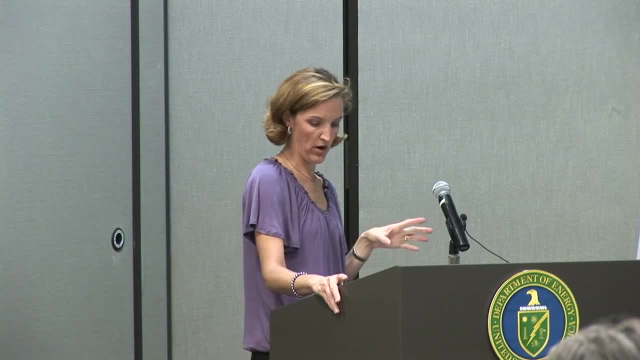 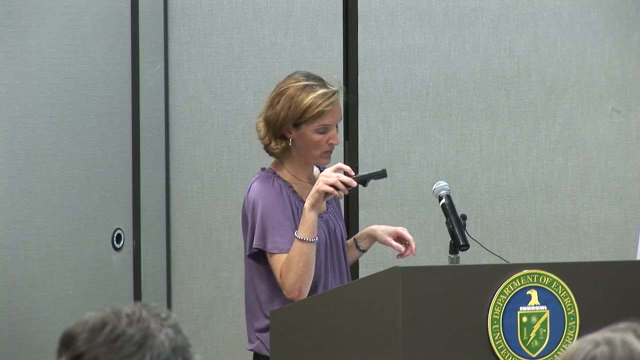 and basically, as we see, the dissolved water reduces the acid yields in the radiolysis. The open circles on here represent the dry TBP and the closed circles represent the water-saturated And, as you see, the water-saturated. 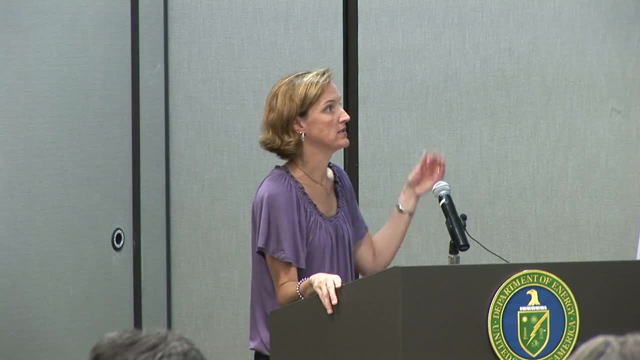 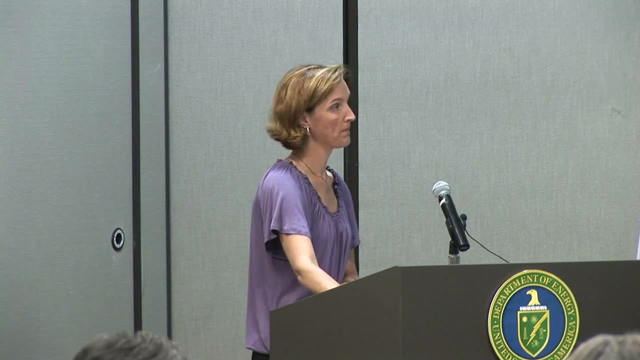 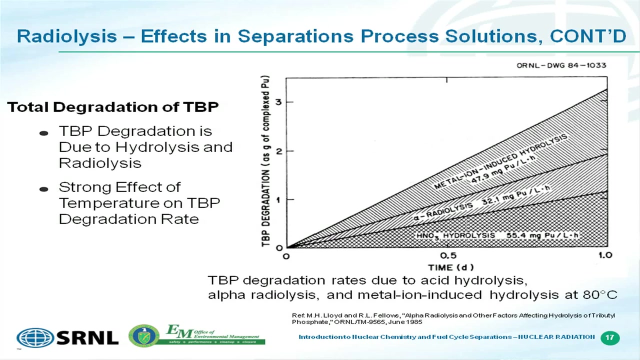 as the TBP concentration increases, the total acid produces a little bit lower than the ones with the dry TBP. TBP breakdown can occur through several mechanisms. This includes hydrolysis as well as radiolysis. This chart basically shows the TBP degradation rates. 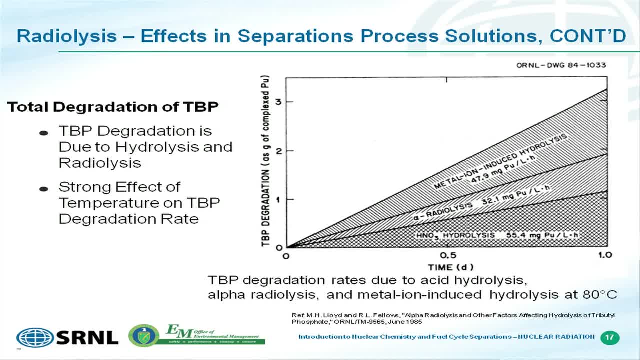 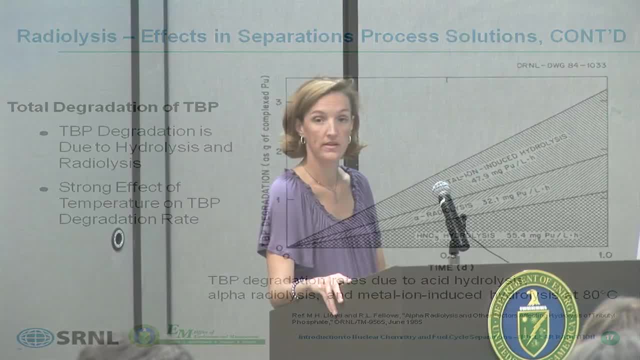 due to acid hydrolysis, alpha-radiolysis and metal-ion-induced hydrolysis at 80 degrees C, And what this shows is the grams of plutonium that are complexed with the degradation products, And the metal-induced hydrolysis does have. a larger effect on the TBP degradation And it is very, very strongly dependent. The chemical hydrolysis, as well as the radiolysis, is very temperature-dependent. Another important process solution that is subject to breakdown in the radiolysis process is hydrolysis. 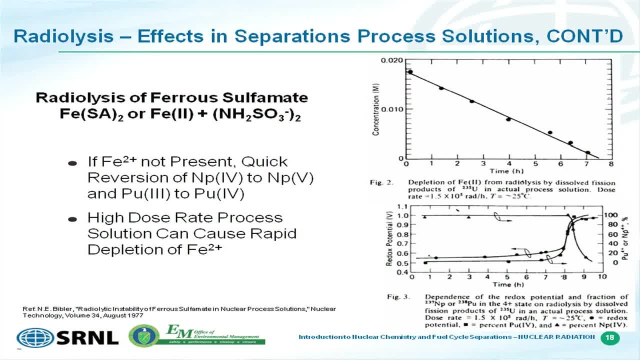 Hydrolysis is a very important process when the breakdown is FSA And, as we said earlier, not FSA. FESA: it acts to reduce and maintain neptunium plutonium in their reduced ionic states. It can be broken down by the radiolytic oxidation of iron. 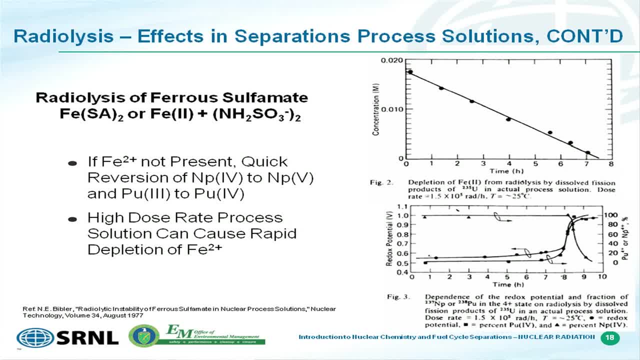 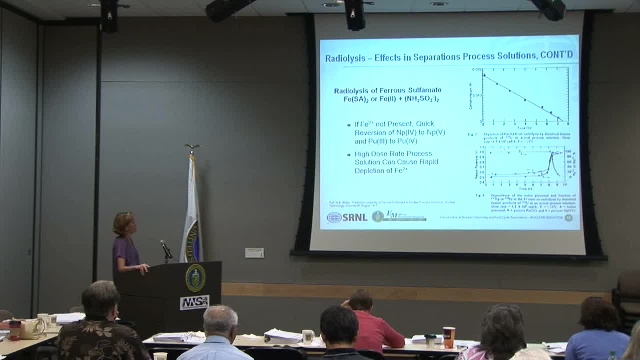 And, as we see in that first chart, when its concentration falls to zero, there's a rapid reversion of the neptunium and the plutonium charge states as shown in the bottom figure. If iron's not present, we see a quick reversion. 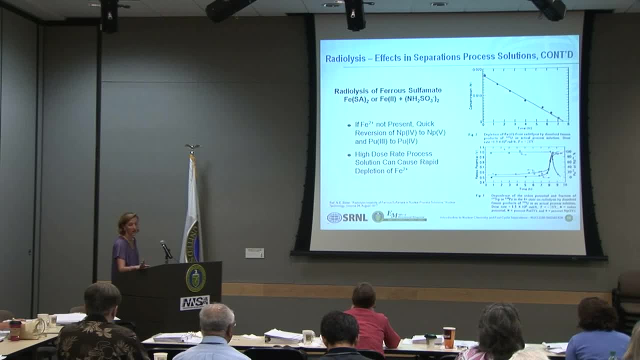 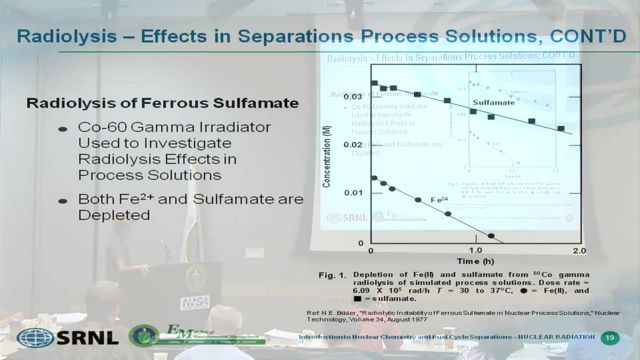 And high dose rates in the process solution cause that rapid depletion. Now Ned Bibler from SRNL did a solid investigation on actual process solutions with its attendant radiation and in simulation testing to demonstrate the utility of using irradiators to investigate radiolysis effects. 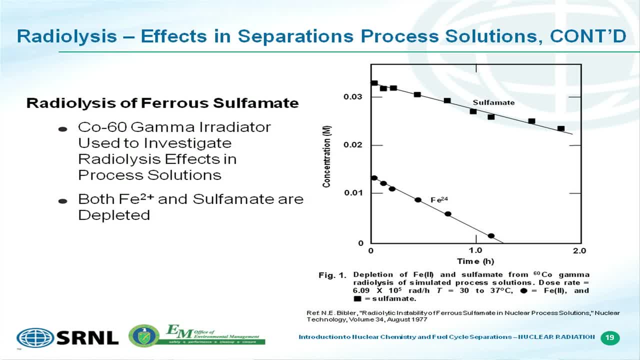 And that's actually what this slide shows. In conjunction with the actual process solutions that we saw in the previous slide, this slide demonstrates that you can use cobalt-60 irradiation to show the effects of the fission products as well. This testing was in our cobalt irradiator. 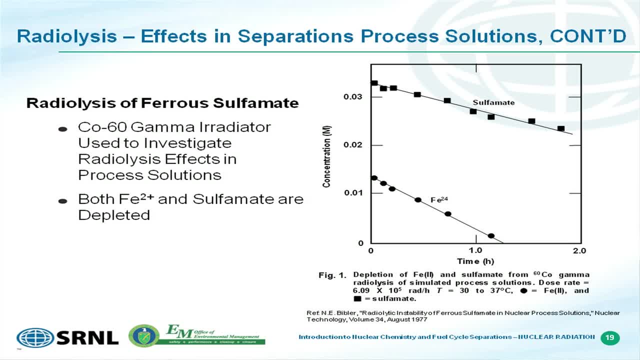 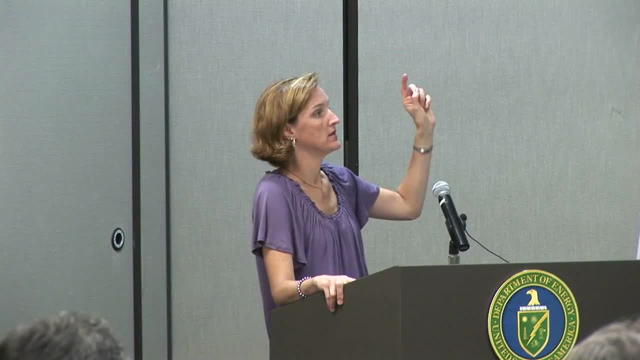 And although it's several times the dose rate of the solution, it is several times the dose rate of the solution with the fission products in the previous slide. But once again it shows, as time goes on, the concentration of iron is depleted with dose. 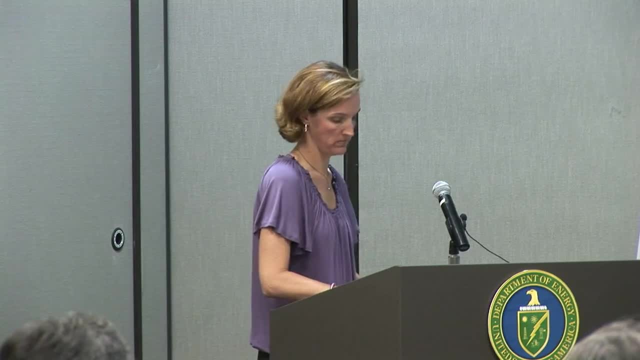 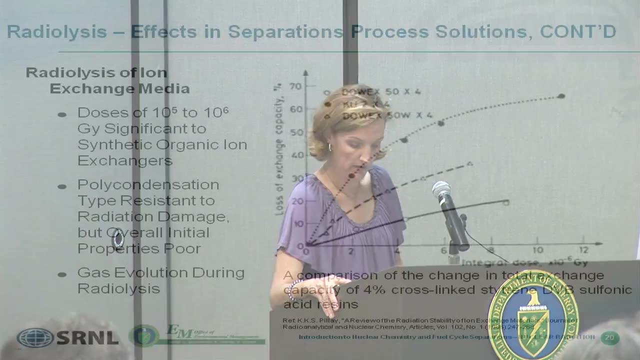 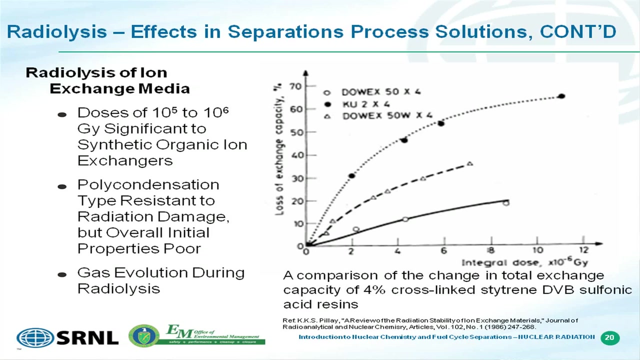 Radiolysis effects has been an empirical science for these process solutions and for the exchange material- The effects of the dose or the energy deposition are reported in terms of generation of breakdown products- and has guided the operations of separations systems. What this shows right here. is, doses of 10 to the 5th to 10 to the 6th gray do significantly reduce the integrity of an organic ion exchanger. And what an organic resin is? basically a high molecular weight polyacid or base that's virtually insoluble. 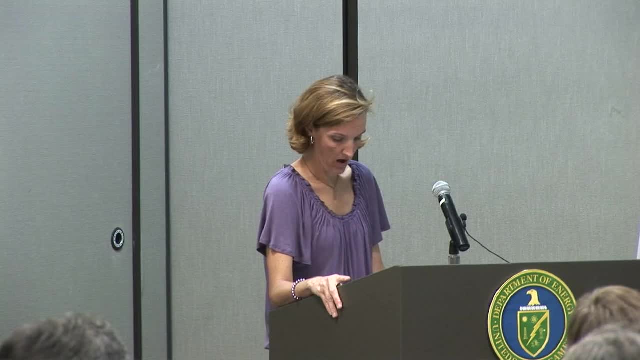 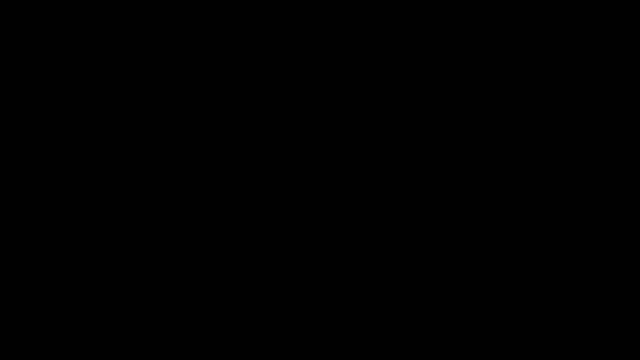 in aqueous and non-aqueous materials, And there are also other factors that might be important to consider for the production of this solution, And here's a quick summary of the results. Here's an example of a sample of the results that we've got so far. 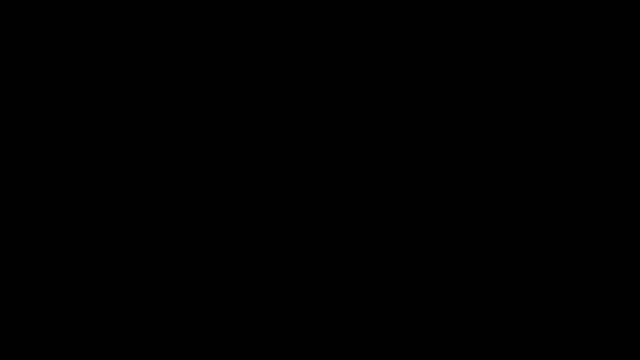 and also what we've seen in the last few slides, And this is a sample of a sample that we've been trying to do with a lot of different solvents. And this is a sample of a sample that we've been trying to do with a lot of different solvents.